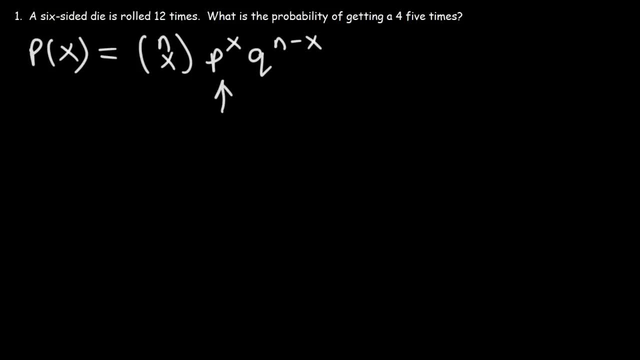 Lowercase p is the probability of getting a success. Lowercase q is the probability that an event fails. So in this problem we need to determine four things: n, x, lowercase p and lowercase q. So what are the values of these four variables? 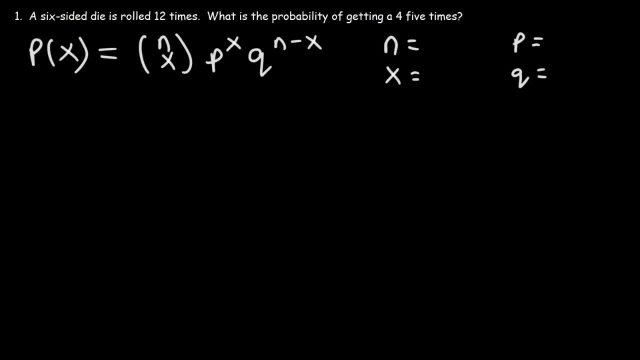 What's n? n is the number of trials. The six-sided die is rolled 12 times, So n is 12.. Now how many successful events are we getting in this problem? We want to get a 4- five times. So we want to successfully get a 4 five times. So there's five successful events. 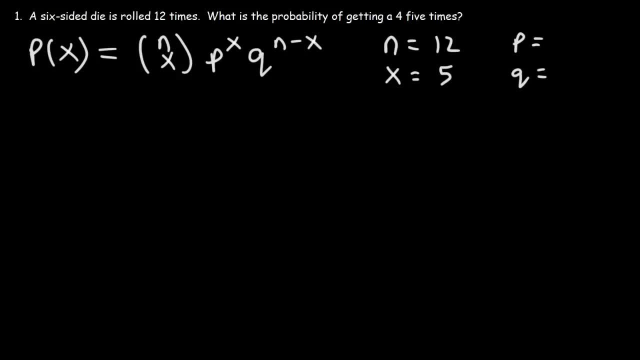 that we're trying to achieve here. Now, what is the probability of getting a successful event? What is the probability of rolling a 4 using a six-sided die? So, out of the six numbers that we can get, there's only one successful number, which? 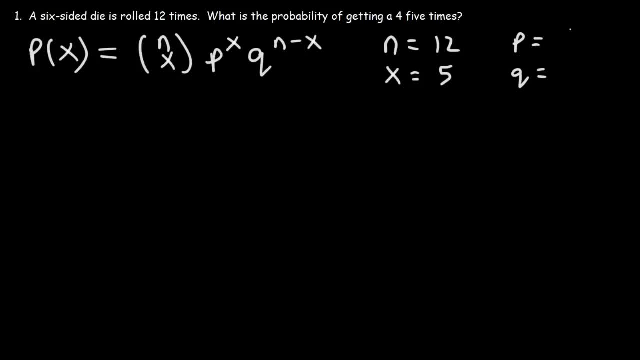 is a 4.. So the probability of rolling a 4 is 1 out of 6, because it's one number out of the six numbers that we can get. Now let's calculate q. What is the probability that the event will fail? What is the probability that we will not get a 4? Out of the six numbers? 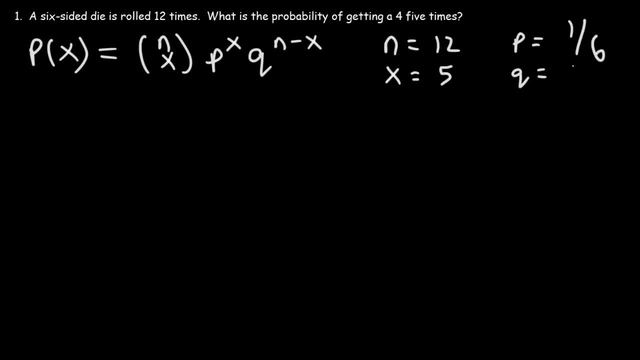 that we can get five of those numbers does not represent a 4.. So the probability of not getting a 4 is going to be 5 out of 6.. Now let's talk about how to calculate this portion of the equation. So we need to use the combination formula. 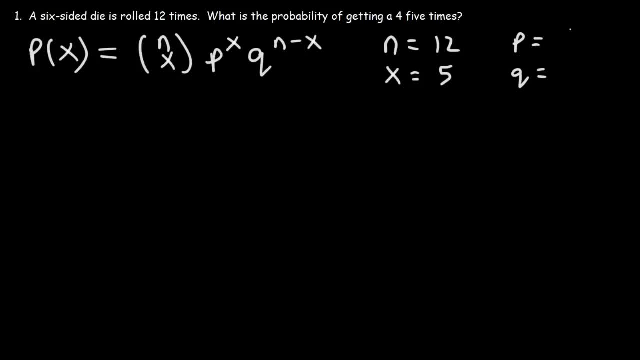 is a 4.. So the probability of rolling a 4 is 1 out of 6, because it's one number out of the six numbers that we can get. Now let's calculate q. What is the probability that the event will fail? What is the probability that we will not get a 4? Out of the six numbers? 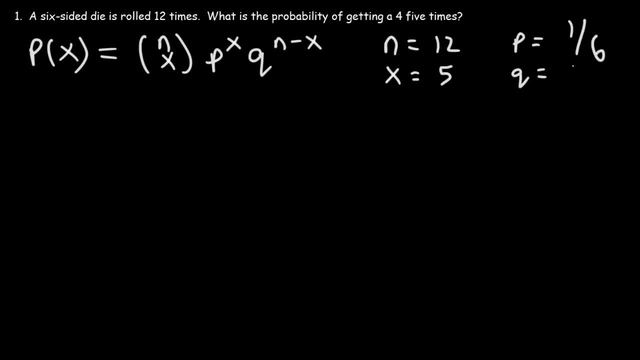 that we can get five of those numbers does not represent a 4.. So the probability of not getting a 4 is going to be 5 out of 6.. Now let's talk about how to calculate this portion of the equation. So we need to use the combination formula. 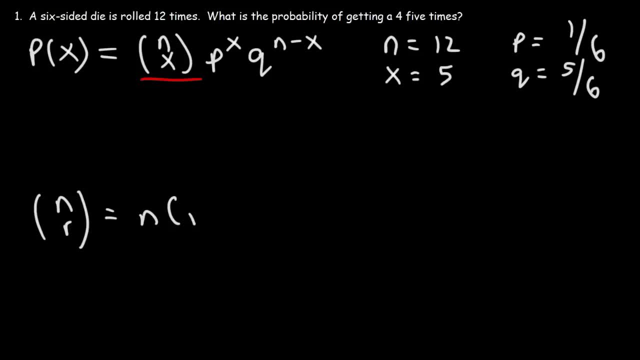 Perhaps you've seen it: This is ncr and that's going to equal n factorial divided by n minus r factorial, times r factorial. So n is 12.. So x is 5.. So this is 12c5.. So that's going to equal 12 factorial divided by 12 minus 5 factorial and then times r. 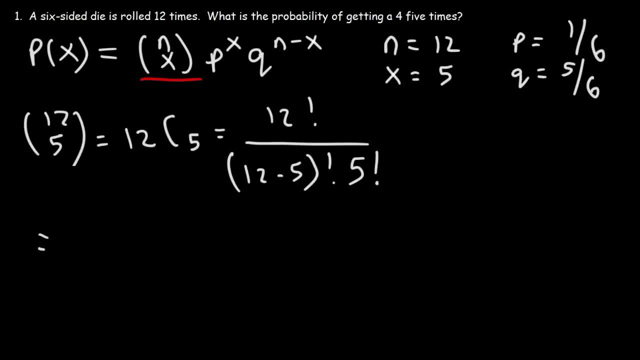 factorial or 5 factorial, 12 factorial, That's going to be 12 times 11.. 12 times 11. Times, 9. Times, 9.. All the way to: 1. Times, 8. Times, 7 factorial. 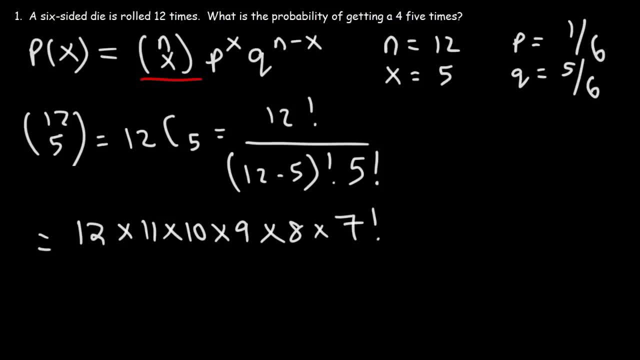 7 factorial is basically 7 times 6 times 5 times 4 times 3 times 2 times 1.. Now 12 minus 5 is 7.. So we can write that as 7 factorial. Note that we can cancel these two. 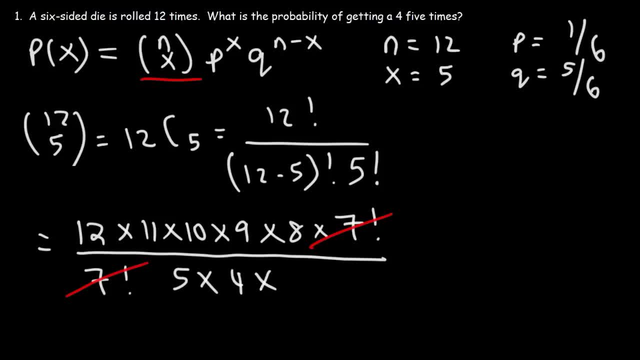 5 factorial. That's going to be 5 times 4 times 3 times 2 times 1.. 5 times 4 times 3 times 2 times 1.. 5 factorial times 2 times 1.. Now 4 and 3, they multiply to 12, so we can cancel that with the 12 on top. 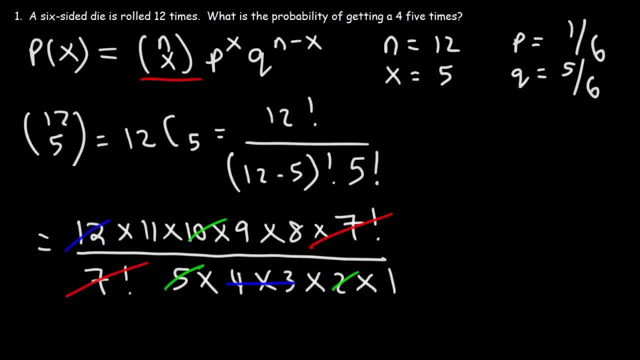 5 times 2 is 10.. So what we have left over is 11 times 9 times 8.. 11 times 9 is 99.. 99 times 8 is 792.. So this portion of the formula is equal to 792.. 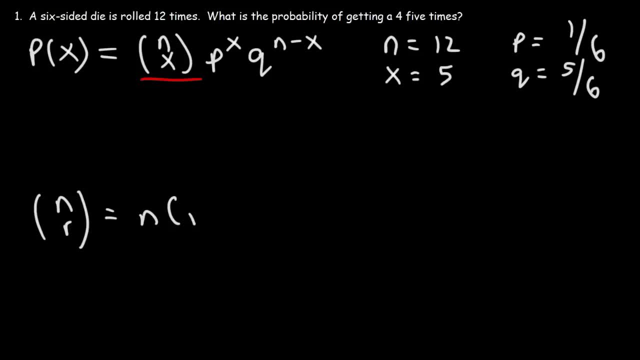 Perhaps you've seen it: This is ncr and that's going to equal n factorial divided by n minus r factorial, times r factorial. So n is 12.. So x is 5.. So this is 12c5.. So that's going to equal 12 factorial divided by 12 minus 5 factorial and then times r. 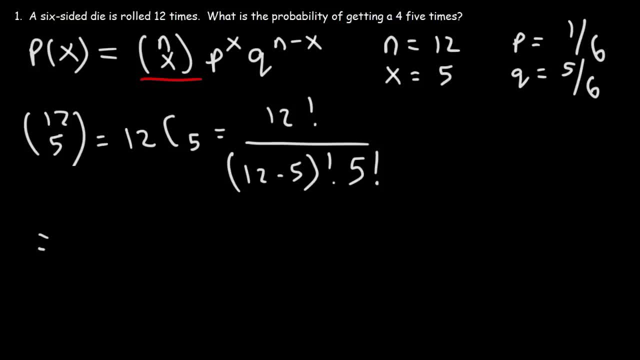 factorial or 5 factorial, 12. factorial, That's going to be 12 times 11.. That's going to be 12 times 10 times 9, all the way to 1, times 8 times 7. factorial, 7- factorial is basically 7 times 6 times 5 times 4 times 3 times 2 times 1.. 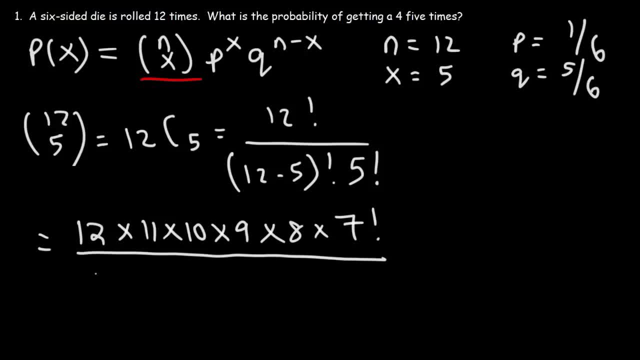 Now 12 minus 5 is 7.. So we can write that as 7 factorial And note that we can cancel these two 5 factorial That's going to be 5 times 4 times 3 times 2 times 7.. 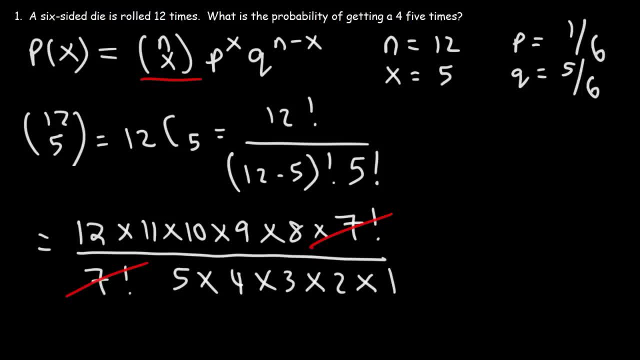 5. times 2 times 1.. Now 4 and 3, they multiply to 12, so we can cancel that with the 12 on top. 5 times 2 is 10.. So what we have left over is 11 times 9 times 8.. 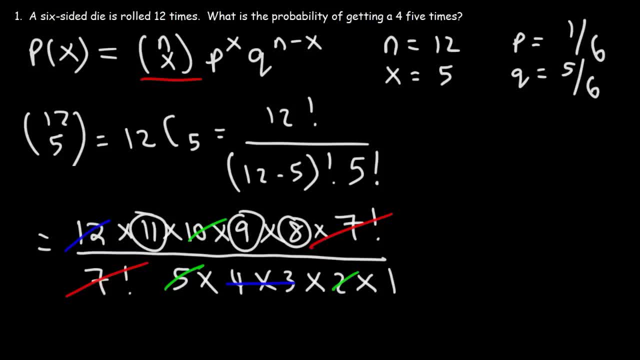 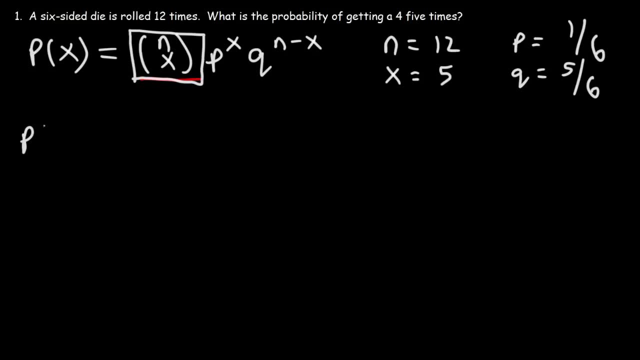 11 times 9 is 99.. 99 times 8 is 792.. So this portion of the formula is equal to 792.. So we have p of x where x is 5.. That's equal to 792 times lowercase p, which is 1 over 6,. 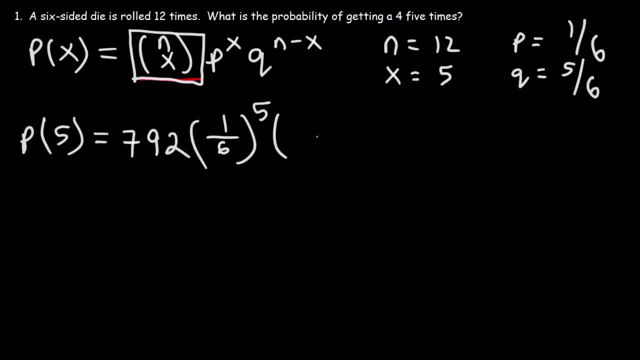 raised to the x power or to the fifth power times q, which is 5 over 6,. raised to the x power or to the fifth power times q, which is 5 over 6, and minus x or 12 minus 5.. 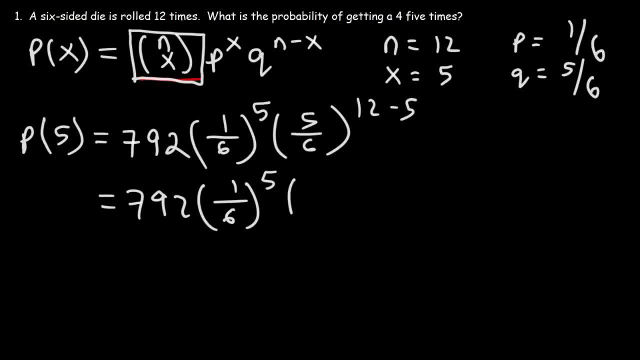 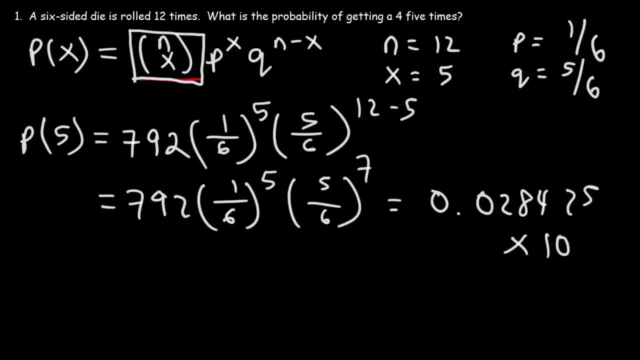 0.0284. 0.0284. 0.0284. 0.0284. 0.0284. 0.0284.. If we multiply that by 100%, we're going to get approximately 2.84%. 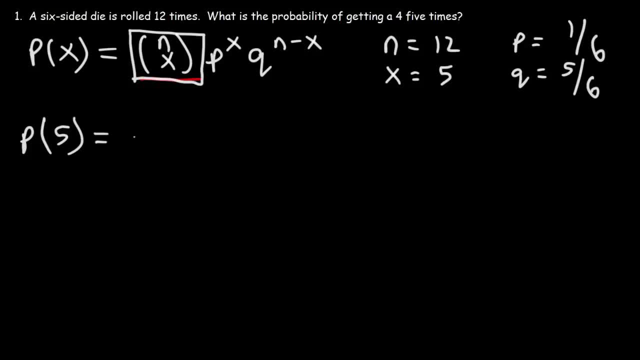 So we have P of X where X is 5.. That's equal to 792 times lowercase p, which is 1 over 6, raised to the X power or to the fifth power times Q, which is 5 over 6,. 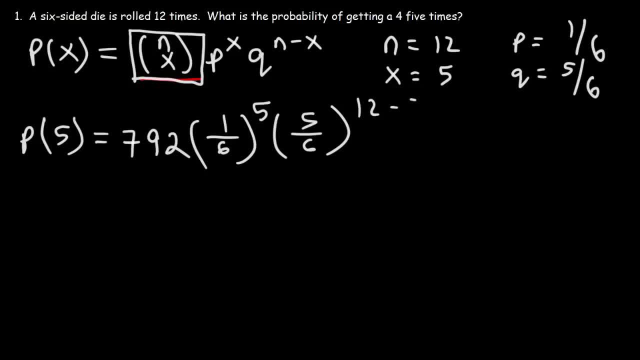 raised to the X power: n minus x or 12 minus 5.. So at this point you can just plug this in to your calculator and get the answer. So just type it exactly the way you see it, And so you should get .028425.. 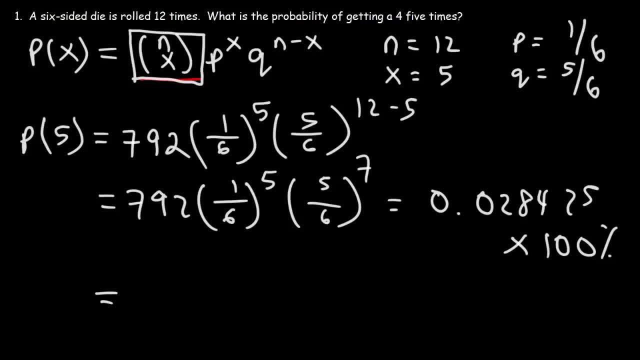 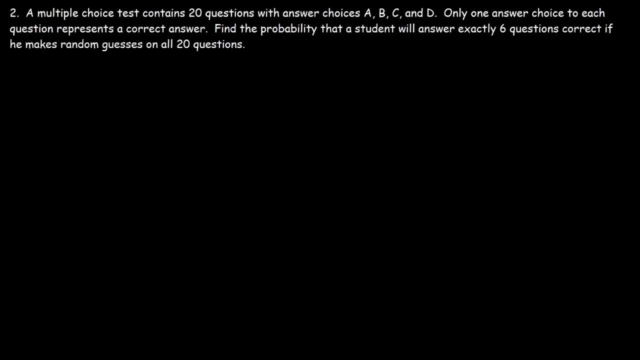 If we multiply that by 100%, we're going to get approximately 2.84%. So that's the probability of getting a 4- 5 times. if we roll a 6 sided die 12 times Number 2.. A multiple choice test contains 20 questions. 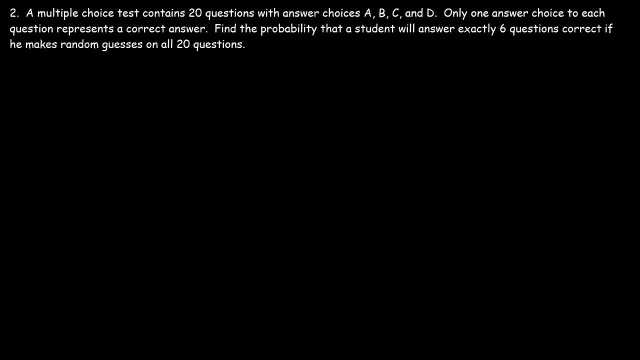 With answer choice 2. And a multiple choice 3. And a multiple choice 3. And a multiple choice 4. And a multiple choice 5. And a multiple choice 4.. This is A, B, C and D. Only one answer choice to each question represents a correct answer. 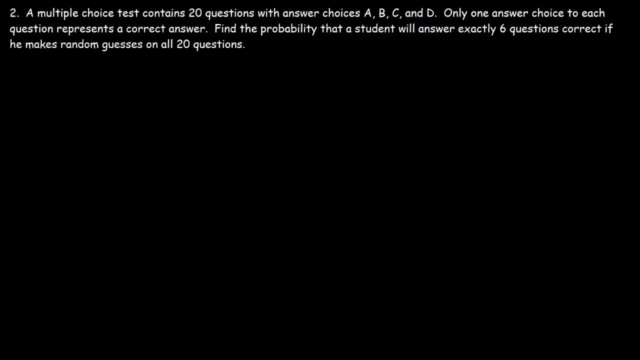 Find a probability that a student will answer exactly 6 questions correct if he makes random guesses on all 20 questions. So go ahead and take a minute and try this problem. So let's begin with the formula. So it's going to be ncx times the probability that it will be successful, raised to the x. 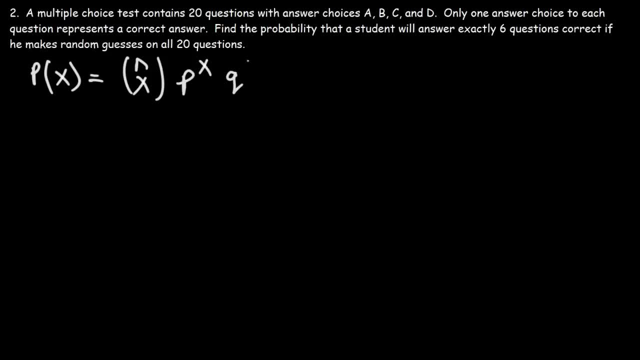 power times, the probability that it's going to fail raised to the n minus x. Now, what are the variables n, x, p and q in this problem? So, like before, n is the number of trials, in this case the 20 questions. 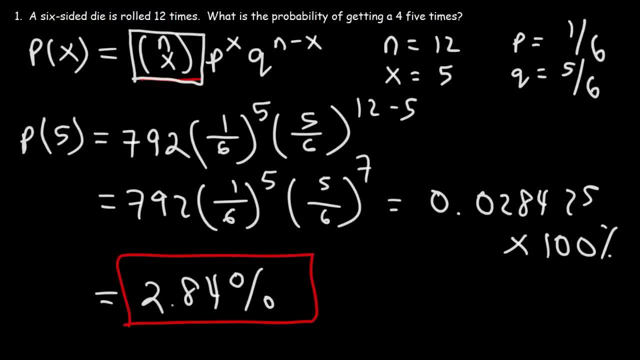 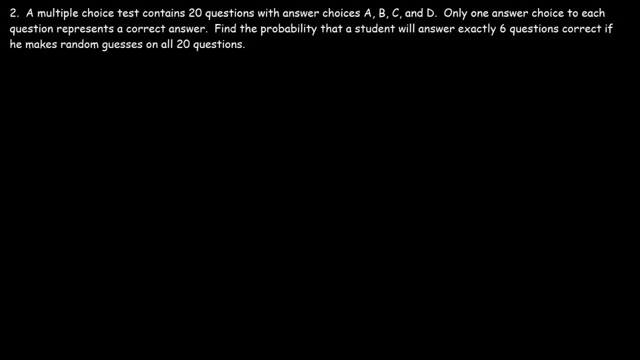 So that's the probability of getting a 4 five times if we roll a six-sided die 12 times. Number two, a multiple choice test, contains 20 questions with answer choices A, B, C and D. Only one answer choice to each question. 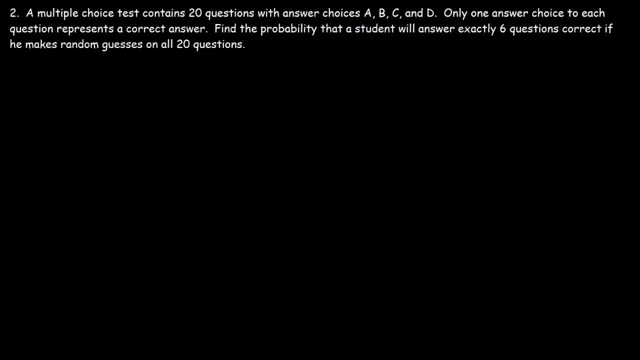 represents a correct answer. Find a probability that a student will answer exactly six questions correct if he makes random guesses on all 20 questions. So go ahead and take a minute and try this problem. So let's begin with the formula. So it's going to be NCX. 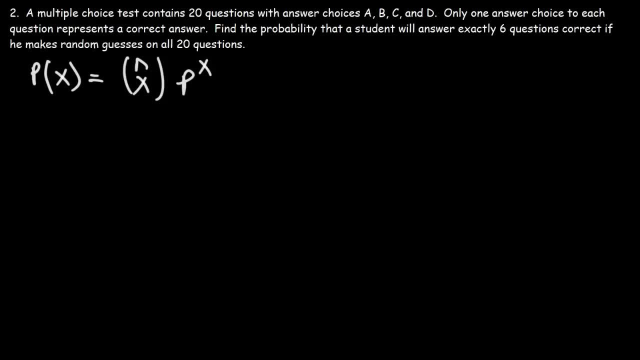 times the probability that it will be successful, raised to the x power times the probability that it's going to fail, raised to the n minus x. Now, what are the variables n, x, p and q in this problem? So, like before, n is the number of trials, in this case the 20 questions. 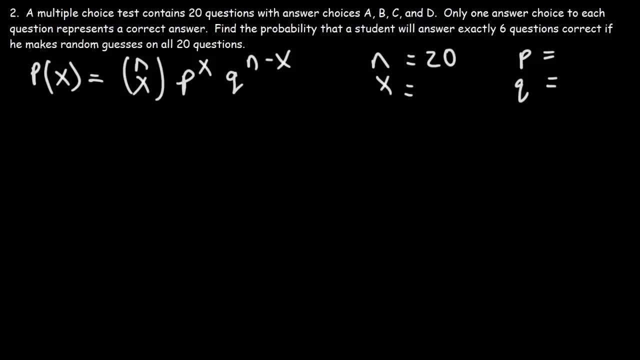 Now, how many of these variables are going to be correct? How many of these 20 trials does a student have to get a successful event? He needs to answer exactly six questions correct out of the 20 questions. So there has to be six successes in 20 trials. Now what are the values of p and q? 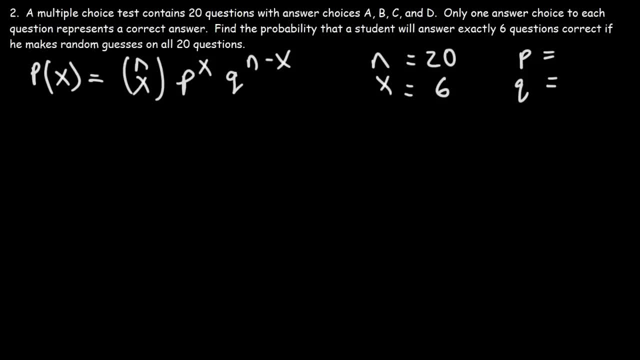 In this case, p is going to be the probability of getting a question right by randomly guessing an answer. So there has to be six successes in 20 trials. So there's four answer choices. one of them is correct, So the probability is going to be one. 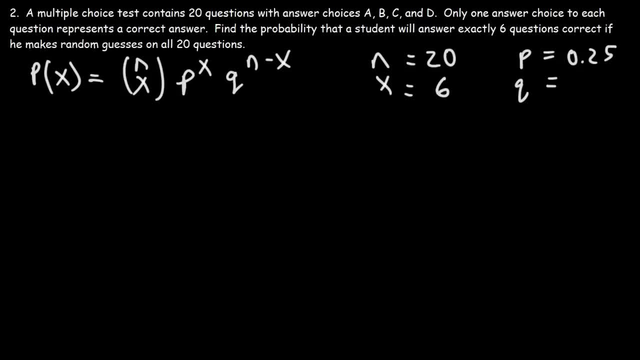 out of four or 0.25, which means the probability of guessing the question wrong is going to be three out of four, because there's only one correct answer. the other three are wrong. Three out of four is basically 0.75.. That's the probability that. 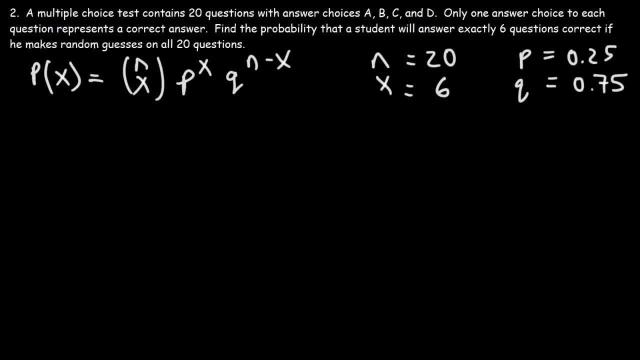 he will get the question wrong if he guess randomly. So now that we have the values of n, x, p and q, Let's go ahead and calculate the value of NCX or 20C6.. This is going to be 20 factorial divided by 20, minus 6 factorial times 6 factorial. 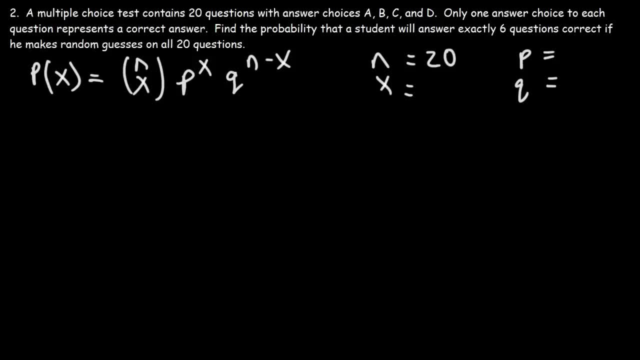 Now how many of these 20 trials does the student have to get a successful event, He needs to answer exactly 6 questions correct out of the 20 questions. So there has to be 6 successes in 20 trials. Now what are the values of p and q? 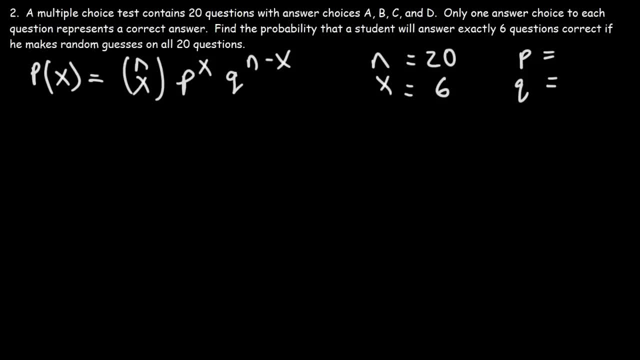 In this case, p is going to be the probability of getting a question right by randomly guessing an answer. So there's 4 answer choices. One of them is correct. So the probability is going to be 1 out of 4, or 0.25, which means the probability of 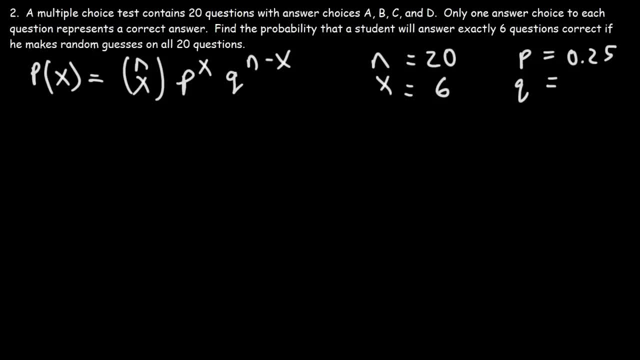 guessing the question wrong is going to be 3 out of 4, because there's only one correct answer. the other 3 are wrong. 3 out of 4 is basically 0.75.. That's the probability that he will get the question wrong if he guesses randomly. So now that we have the values of p and q, we're going to take a look at the probability of getting a question right by randomly guessing an answer. So now that we have the values of p and q, we're going to take a look at the probability. 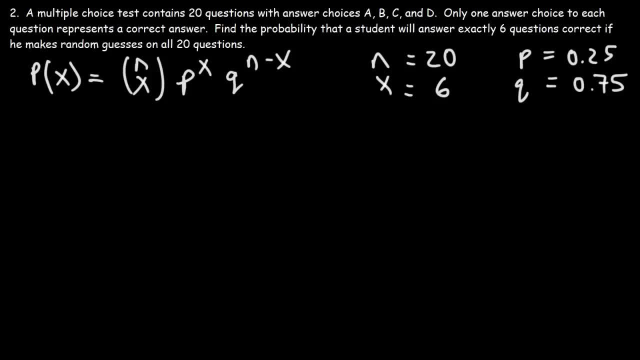 of getting a question right by randomly guessing an answer. So now that we have the values of n, x, p and q, let's go ahead and calculate the value of ncx or 20c6.. This is going to be 20 factorial divided by 20, minus 6 factorial times 6 factorial. 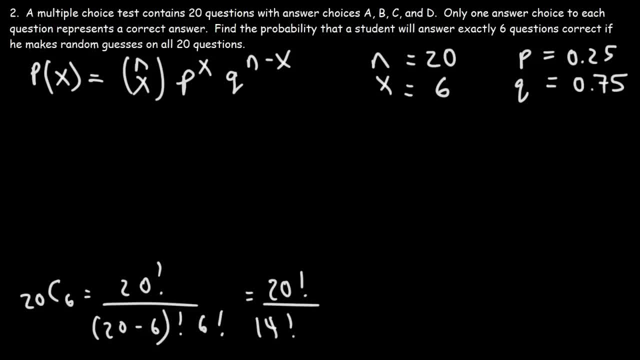 So that's 20 factorial over 20 minus 6 is 14, and then times 6 factorial, So 20 factorial is going to be 20c6.. So 20 times 19, times 18, and we're going to keep going until we get to 14.. 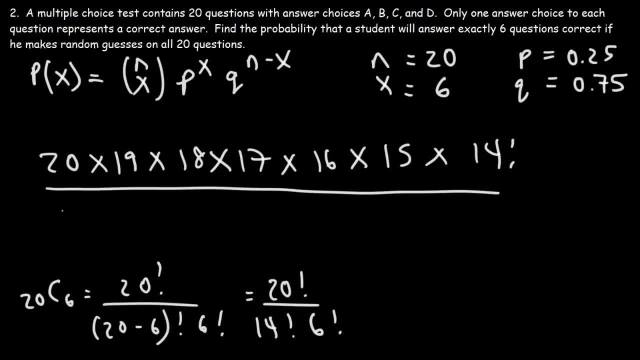 I'm going to leave it as 14 factorial and then I'm going to expand 6 factorial. So we're going to do just like we did before in the previous problem: We're going to cancel 14 factorial and let's see what else we can do. 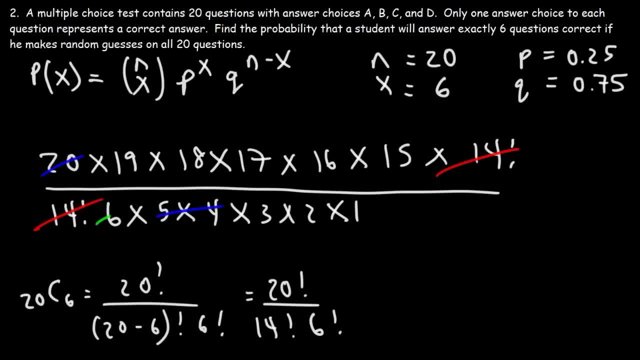 So 5 times 4 is 20.. And 6 times 3, that's going to be 18.. And then 16 divided by 2 is 8.. So what we have now is 19 times 17 times 8 times 15.. 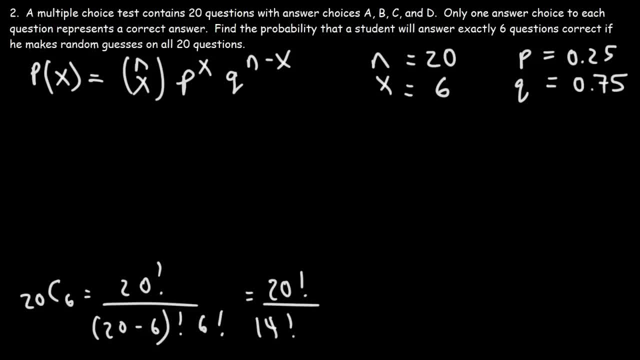 So that's 20 factorial over 20 minus 6 is 14, and then times 6 factorial, So 20 factorial is going to be 20 times 19, times 18, and we're going to keep going until we get to 14.. 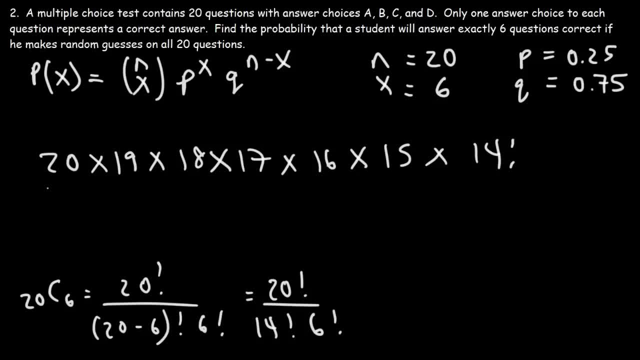 I'm going to leave it as 14 factorial and then I'm going to expand 6 factorial. So we're going to do just like we did before in the previous problem: We're going to cancel 14 factorial and let's see what else we can do. 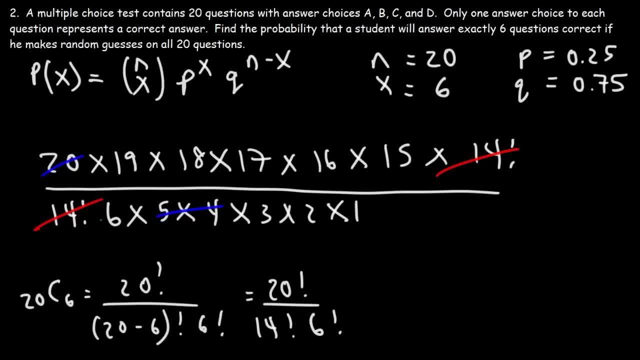 So we're going to cancel 14 factorial and let's see what else we can do. So 5 times 4 is 20 and 6 times 3, that's going to be 18.. And then 16 divided by 2 is 8.. 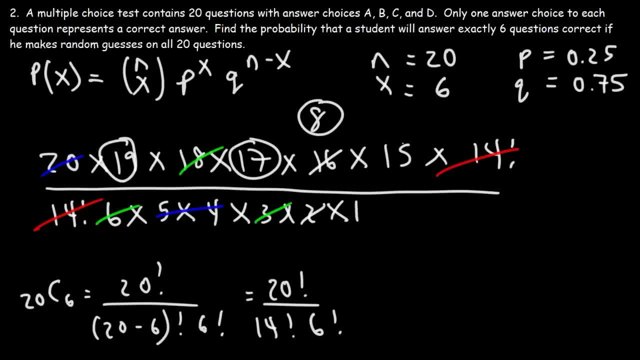 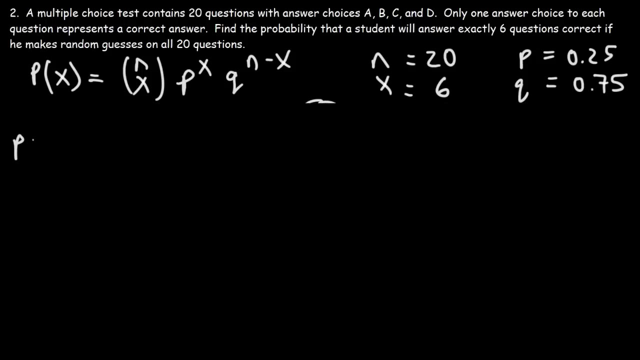 So what we have now is 19 times 17 times 8 times 15.. So if we multiply those four numbers we're going to get 38,760.. Now let's calculate the probability of guessing six answers or six questions correct out of. 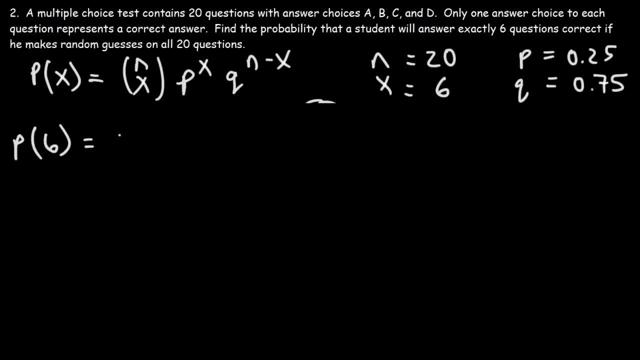 the 20 questions, So it's 20C6, which we got it to be 38,760 times P. P is 0.25, X is 6 times Q, which is 0.75. raised to the N minus X, That's 20 minus 6, which is 14.. 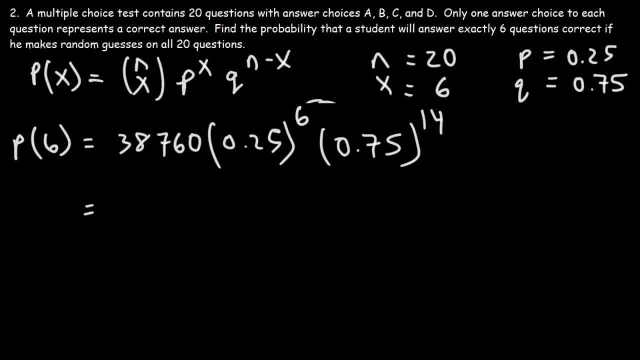 So go ahead and plug in. go ahead and plug those numbers in. I made a mistake. I got to re-type everything. The answer I got is 0.168609.. So I'm going to re-type everything. The answer I got is 0.168609.. 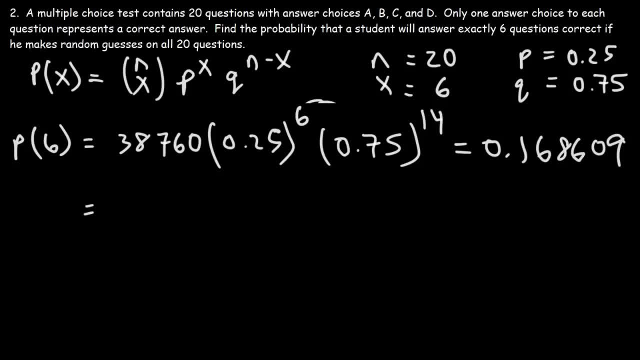 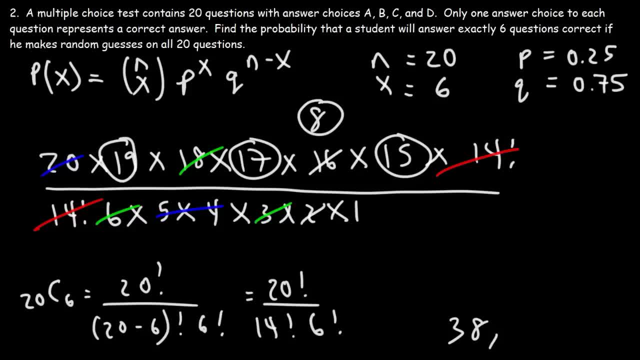 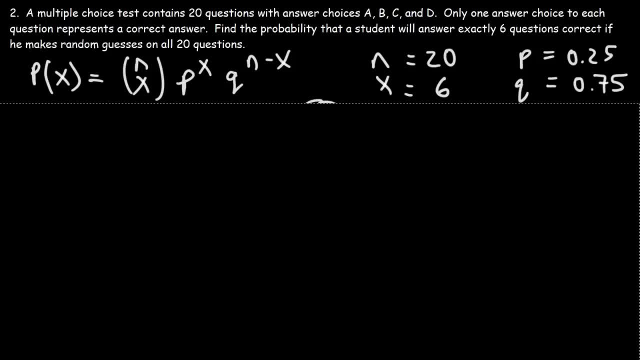 So if we multiply those four numbers, we're going to get 38,760.. Now let's calculate the probability of guessing six answers or six questions correct out of the 20 questions. So it's 20c6, which we got it to be 38,760, times p. 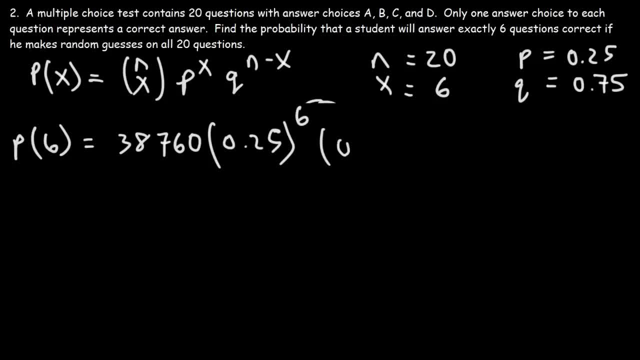 p is 0.25, x is 6, times q, which is 0.75,. raised to the n minus x, That's 20 minus 6,, which is 14.. So go ahead, Go ahead and plug in. 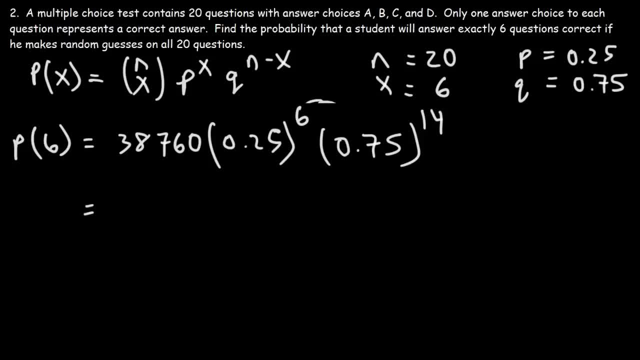 Go ahead and plug those numbers in. I made a mistake. I got to retype everything. The answer I got is 0.168609.. Multiplying that by 100. That's approximately 16.86%. So that's the probability of guessing six questions correct out of the 20 multiple choice. 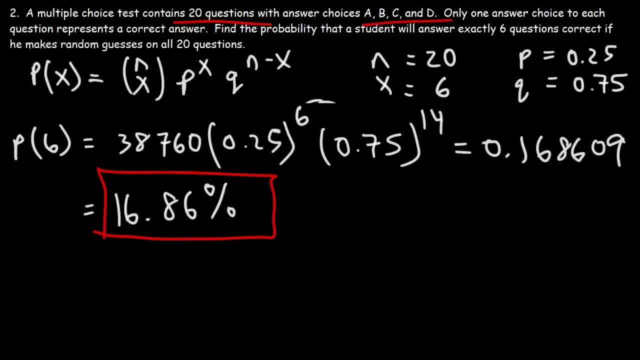 question tests, assuming there's four answer choices. If there were five answer choices, p and q will be different. If there were five answer choices, p would be 0.20, q would be 0.80.. It'll be 1 out of 5 for p. 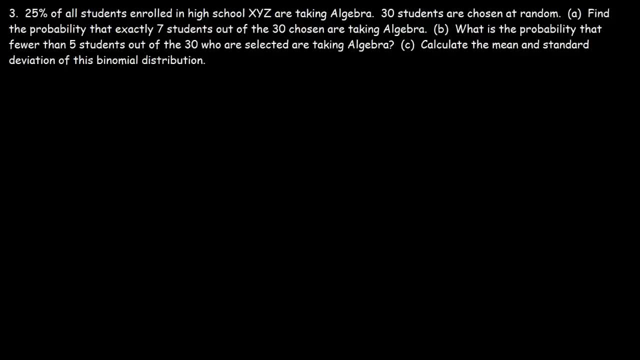 Number 3. 25% of all students enroll in college. That's approximately 16.86%. That's the probability of guessing 6 questions correct out of the 20 multiple choice question tests. Number 4. 30 students enrolled in high school XYZ are taking algebra. 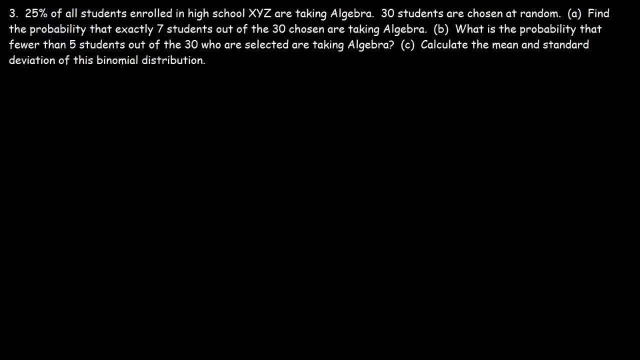 30 students are chosen at random, Part 8. Find the probability that exactly 7 students out of the 30 chosen are taking algebra. Go ahead and work on this problem. So we're going to use the same formula as we've been using in the last two problems. 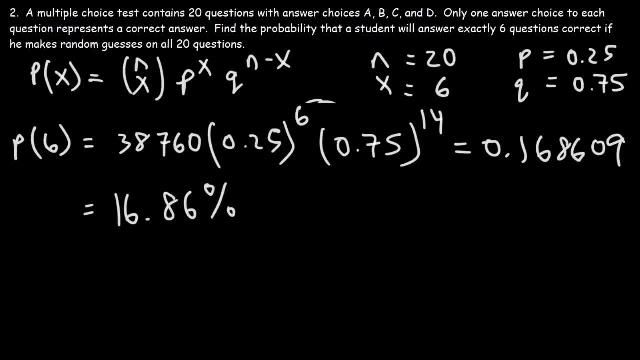 Multiplying that by 100, it's approximately 16.86%. So that's the probability of guessing six questions correct out of the 20 multiple choice question tests, assuming there's four answer choices. If there were five answer choices, P and Q will be different. 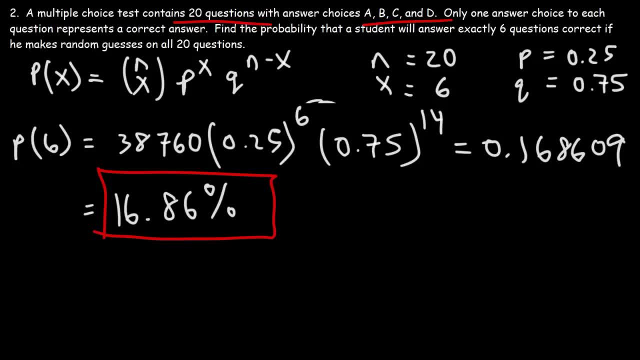 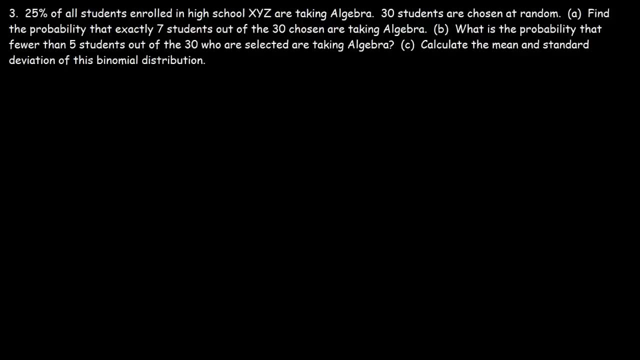 If there were five answer choices, P would be 0.20, Q would be 0.80.. It would be 1 out of 5. for P Number three. All students enrolled in high school x, y, z are taking algebra. 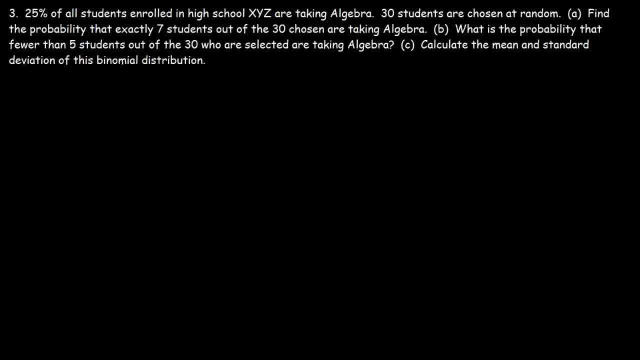 All students enrolled in high school x, y, z are taking algebra. Thirty students are chosen at random Part eight. Find the probability that exactly seven students out of the 30 chosen are taking algebra. Go ahead and work on this problem. 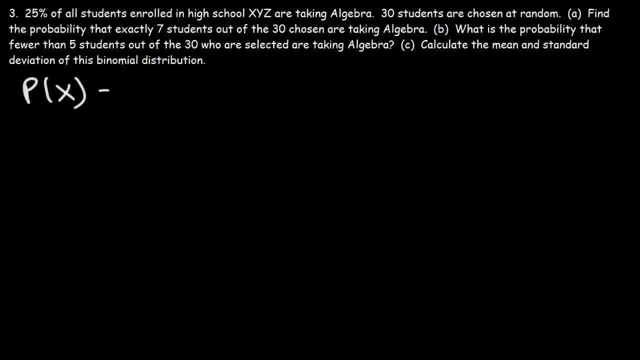 We're going to use the same formula as we've been using in the last 20 questions: Okay problems. So what is N in this problem? N is going to be the number of students that are chosen at random, That's 30.. X is going to be the number of successes in N trials. So these are going to be. 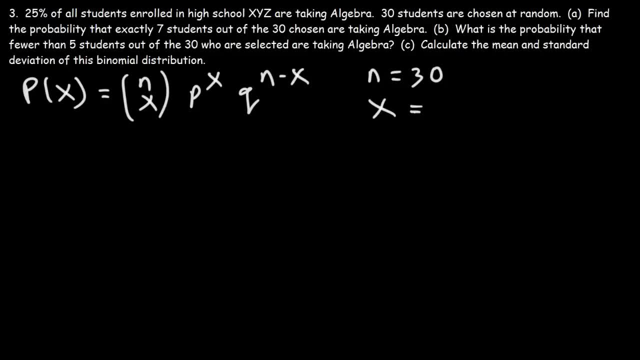 the number of students who are taking algebra out of the 30 chosen. So X is going to be 7.. P is the probability of selecting a student who is taking algebra, and that's going to be 25% or 0.25.. The probability of selecting a student who is not taking algebra. that's going to be Q. 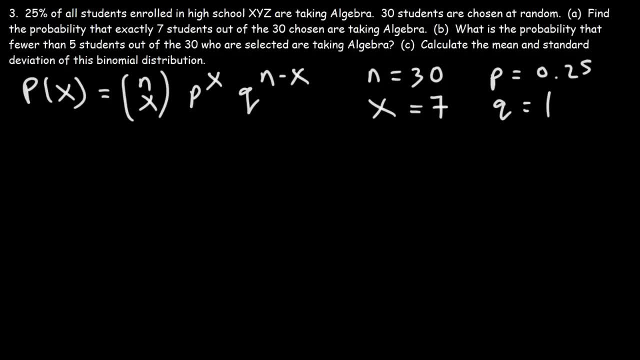 which is 1 minus P, which is 1 minus 0.25, and that's 0.75.. So now we have everything that we need to answer part A. So we need to calculate P of 7.. So this is going to be 30 and 7 times 0.25 raised to the 7th power. 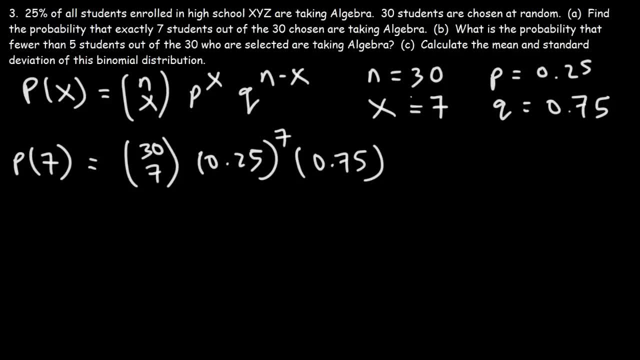 times 0.75, raised to the 30 minus 7 power. So at this point you know how to use the combination formula to calculate 30 C7.. So I'm just going to use my calculator to get this right. So I'm going. 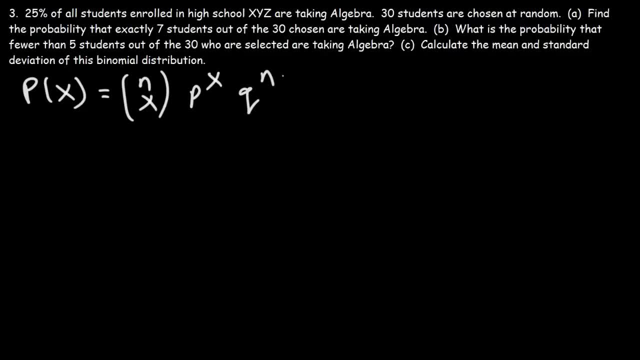 problems. So what is n in this problem? n is going to be the number of students that are chosen at random, That's 30.. x is going to be the number of successes in n trials. So these are going to be the number of students who are taking algebra out of the 30 chosen. So x is going to be 7.. 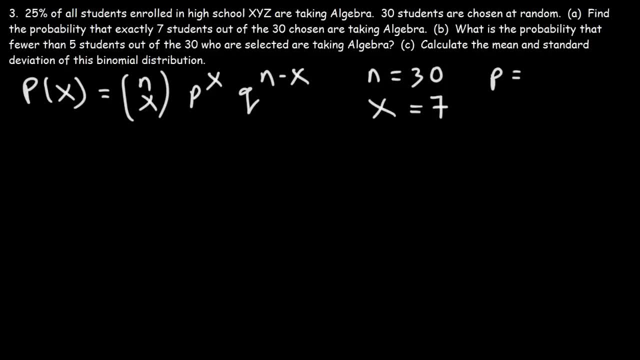 p is the probability of selecting a student who is taking algebra, and that's going to be 25% or 0.25.. The probability of selecting a student who is not taking algebra, that's going to be q, which is 1 minus p, which is 1 minus 0.25, and that's 0.75.. So now we have everything that we. 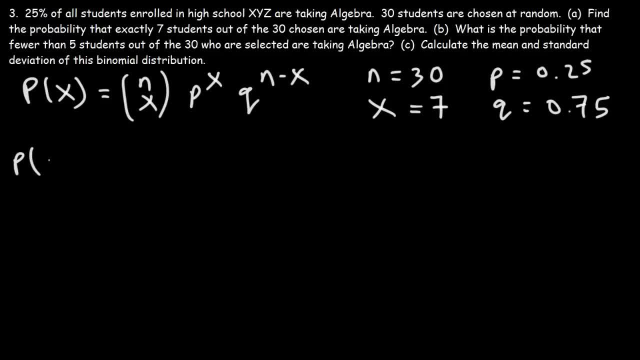 need to answer part a. So we need to calculate the number of successes in n trials. So we need to calculate p of 7.. So this is going to be 30 n7 times 0.25, raised to the 7th power. 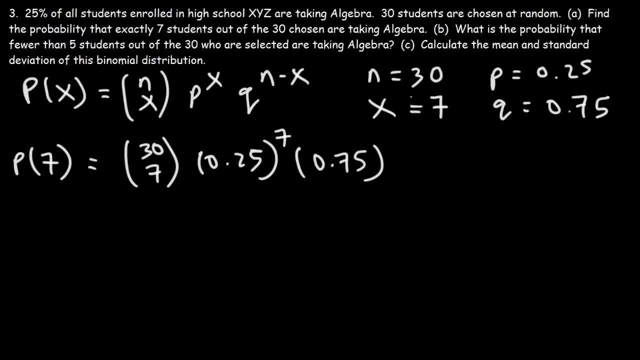 times 0.75, raised to the 30 minus 7 power. So at this point you know how to use the combination formula to calculate 30 c7.. So I'm just going to use my calculator to get this answer: 30 c7, that is a huge number, It's 2,035,800. 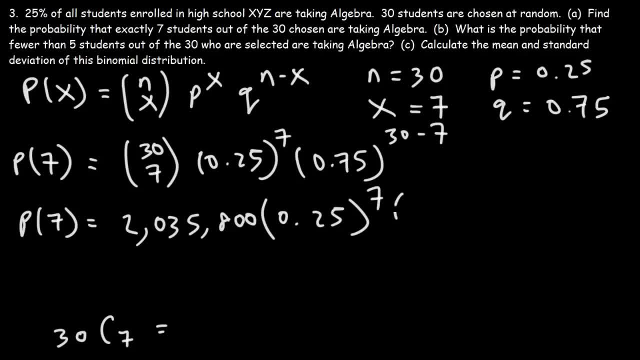 We're going to multiply that by 0.25 raised to the 7th, times 0.75 raised to the 23rd power, So the answer is going to be 0.167.. If we multiply that by 100%, the answer is approximately 16.6%. 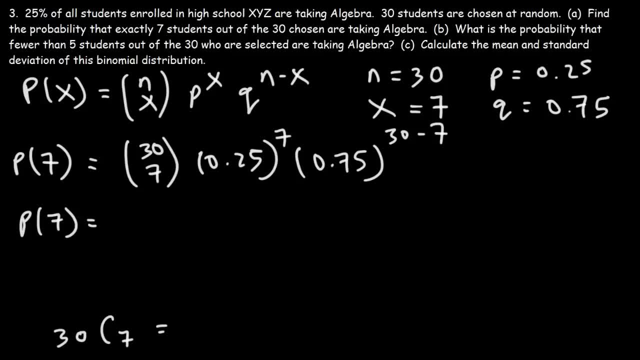 to use this answer: 30 C7, that is a huge number, It's 2,035,800.. And we're going to multiply that by 0.25, raised to the 7 times 0.75, raised to the 23rd power. So the answer is going to be: 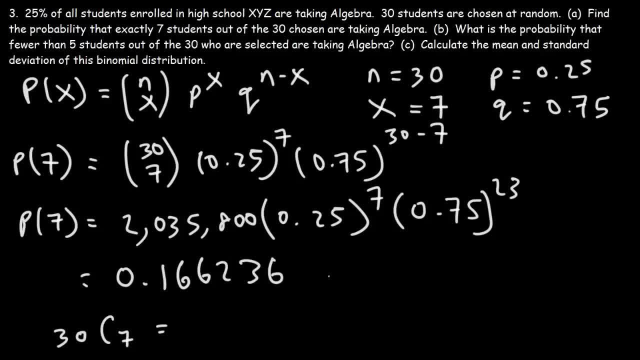 166,236.. If we multiply that by 100%, the answer is approximately 16.6%. So that is the probability of selecting exactly seven students out of 30 who are taking algebra and who are enrolled in this school. Now go ahead and try part B. Feel free to pause the video. 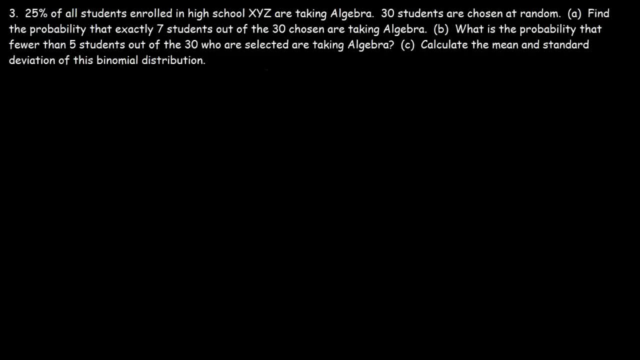 And work on that example. What is the probability that fewer than five students out of the 30 who are selected are taking algebra? So now we're not dealing with just one number, but a range of values for x, So x has to be less than five. 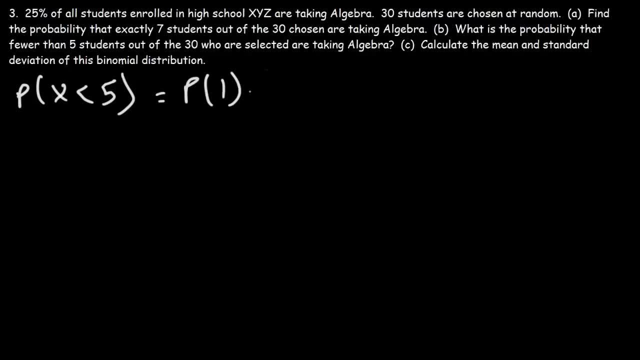 Which means it can be 1,, it can be 2,, 3, or 4,, but not 5.. It's not less than or equal to 5, it's just less than 5.. So what we're going to have to do is calculate the probability when x is 1,, 2,, 3, and 4,. 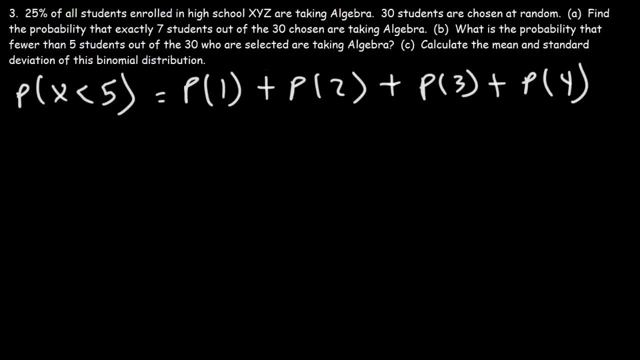 and then add them up in order to get this answer. So let's find the probability that exactly one student out of the 30 is chosen at random who is taking algebra. So n is going to be 1,, 2,, 3, or 4,, but not 5.. So let's find the probability that exactly one student out of the 30 is chosen at random who is taking algebra. 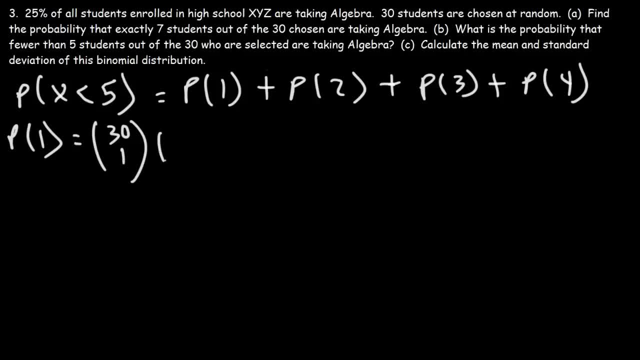 So n is going to be 30, x is 1, p is still the same, it's 0.25.. So it's 0.25 raised to the x, x is 1, q is the same, 0.75 raised to the n minus x, or 30 minus 1, which is 29.. 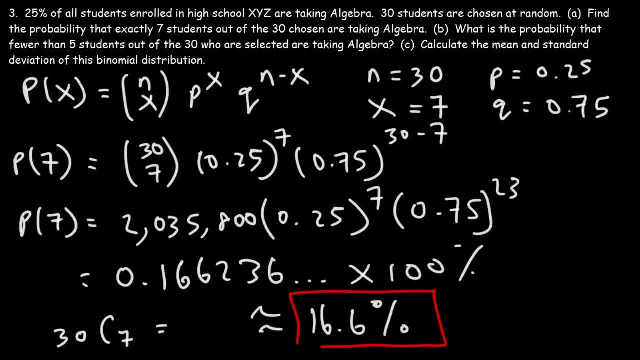 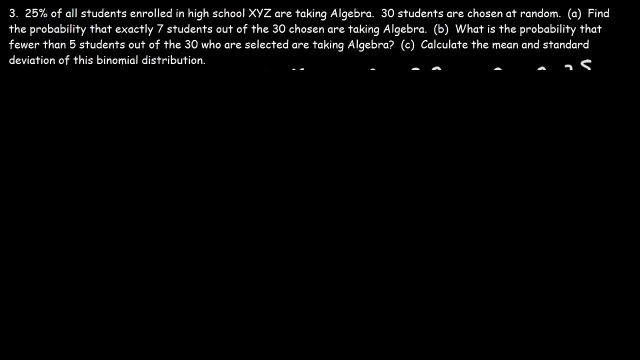 So that is the probability of selecting exactly 7 students out of 30 who are taking algebra and who are enrolled in this school. Now go ahead and try part B. Feel free to pause the video And work on that example. What is the probability that fewer than 5 students out of the 30 who are selected are? 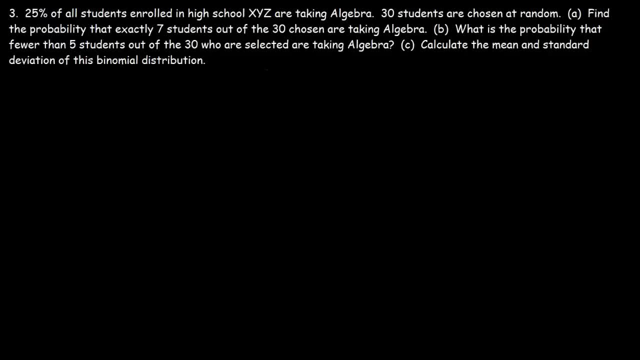 taking algebra. So now we're not dealing with just one number, but a range of values for x. So x has to be less than 5.. Which means it can be 1.. It can be 2,, 3, or 4,, but not 5.. 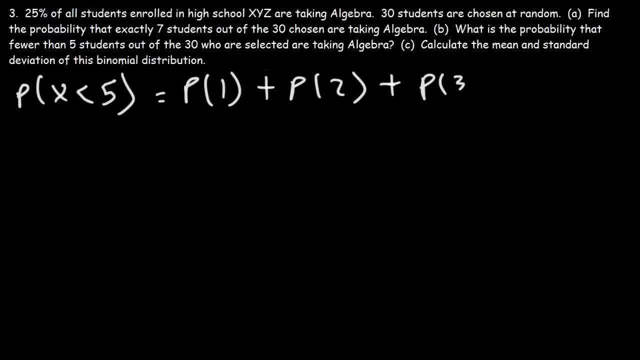 It's not less than or equal to 5,, it's just less than 5.. So what we're going to have to do is calculate the probability when x is 1,, 2,, 3, and 4, and then add them up in order to get this answer. 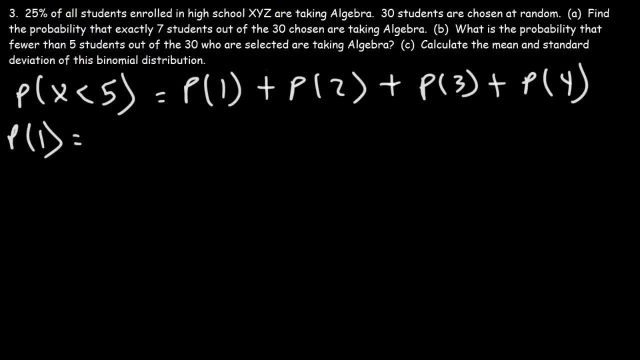 So let's find the probability that exactly one student out of the 30 is chosen at random who is taking algebra. So n is going to be 30, x is 1, p is still the same, it's 0.25.. 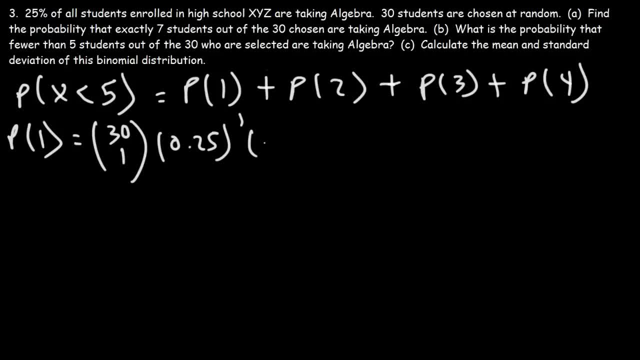 So it's 0.25 raised to the x, x is 1, q is the same, 0.75 raised to the n minus x, or 30 minus 1, which is 29.. So this is going to be 30, c1,. hopefully you have a calculator that can do that times. 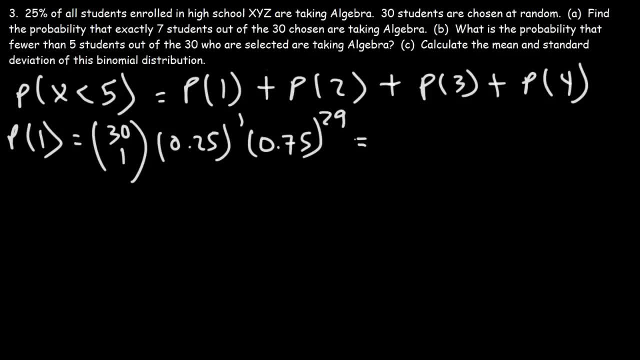 0.25 times 0.75, raised to the 29.. So that's the probability, And so you should get 0.0017858.. Multiplying that by 100, this is approximately 0.1786%. Now let's calculate the probability that, out of the 30 students who are chosen exactly 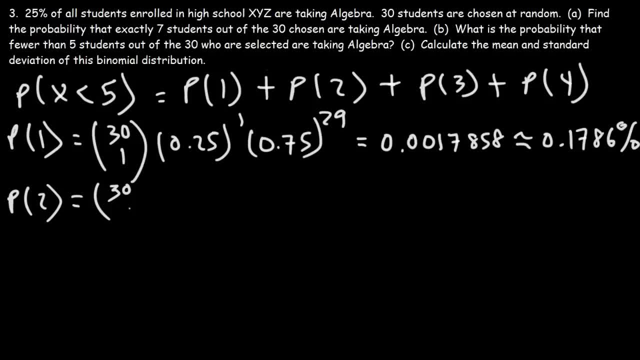 2 are taking algebra, So this is going to be 30, c2.. This is going to be 30, c1, and c2, times 0.25,. raised to the second power, times 0.75,. 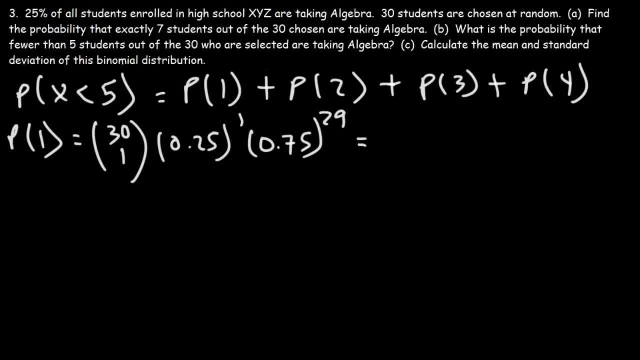 So this is going to be 30, c1, hopefully you have a calculator that can do that- times 0.25, times 0.75, raised to the 29th power, And so you should get 0.0017858.. 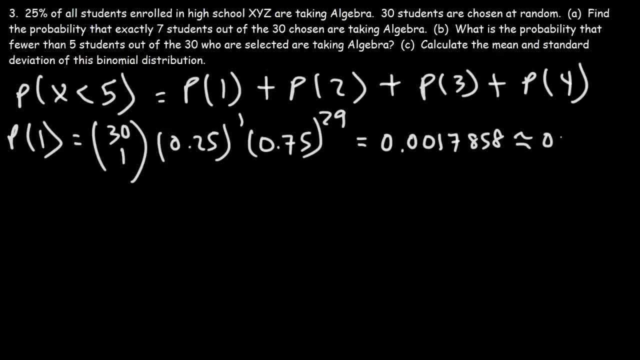 Multiplying that by 100, this is approximately 0.1786%. Now let's calculate the probability that out of the 30 students who are chosen, exactly 2 are taking algebra. So this is going to be 30, c2, times 0.25. 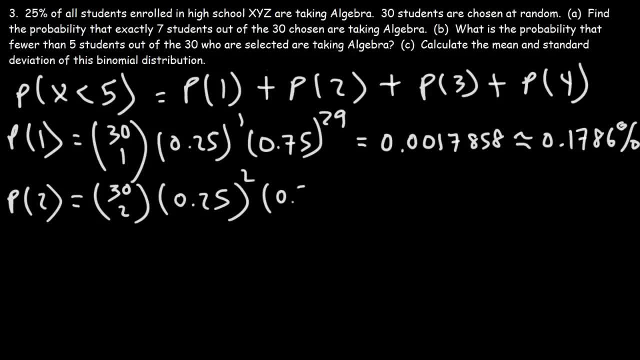 0.25 raised to the 2nd power times 0.75 raised to 30 minus 2, or to the 28th power. So the answer I got for this is 0.0086315.. 0.0086315.. 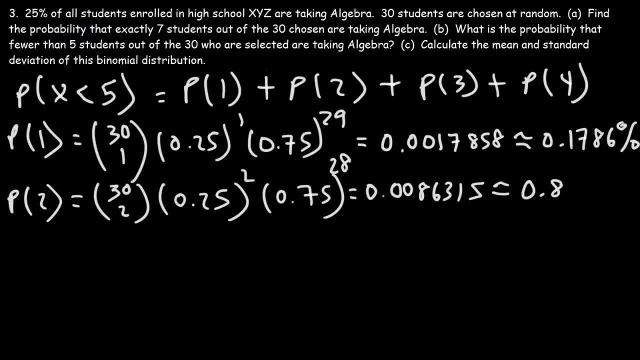 Which is approximately 0.0086315.. 0.8631%- Well, this should be 4.6.. So I'm going to round it to 0.8631.. Now let's calculate p of 3, using the same process. 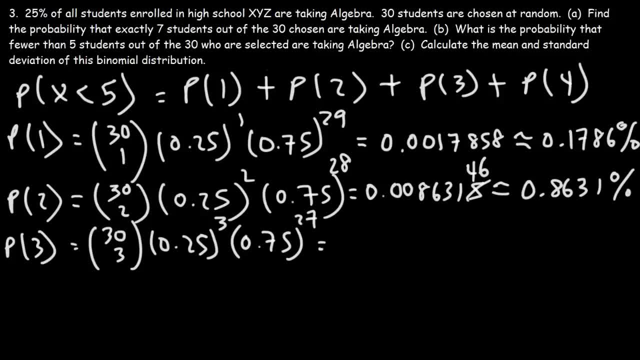 30 minus 3 is 27.. So it's 30, c3, times 0.25, raised to the 3rd power, times 0.75, raised to the 27th power, And this is going to be 0.02685.. 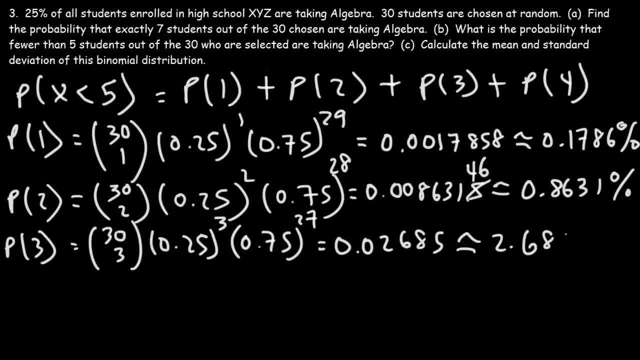 Which is 2.685%. Now let's calculate p of 4.. So it's 30, c4, times 0.25, raised to the 27th power, And this is going to be 0.02685.. 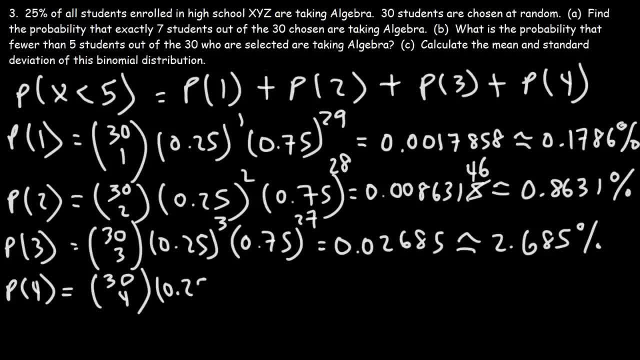 Which is 2.685%. Now let's calculate p of 4.. So it's 30, c4, times 0.0685.. 0.0685%. And then we have to这样: 32 sendo 15, 6.. 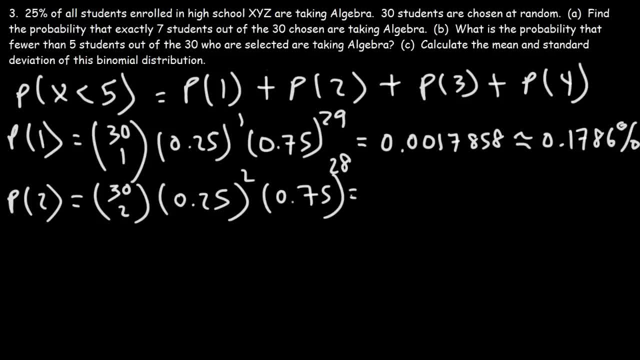 raised to 30 minus 2, or to the 28th power. So the answer I got for this is 0.0086315.. Which is approximately 0.78.. That's it, Thank you Bye. 0.8631%. Well, this should be 4.6, so I'm going to round it to 0.8631.. Now let's calculate. 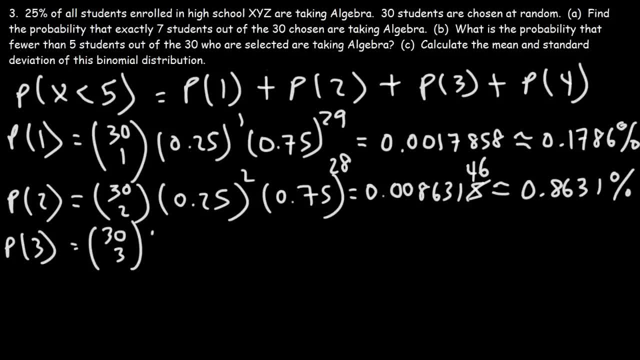 P of 3 using the same process, 30 minus 3 is 27.. So it's 30 C3 times 0.25 raised to the third power, times 0.75 raised to the 27th power, And this is going to be 0.02685, which is: 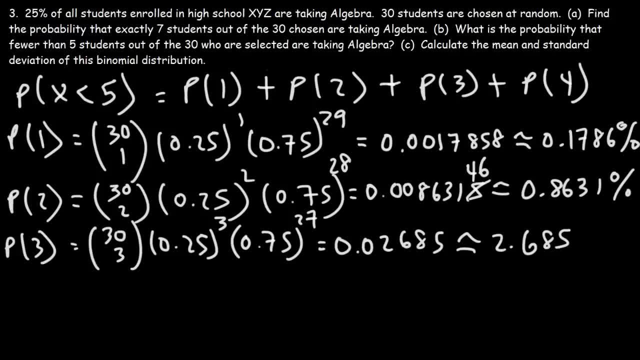 2. 0.2685%. Now let's calculate P of 4.. So it's 30 C4 times 0.25 to the fourth power, times 0.75 to the 26th power. So this comes out to 0.06042.. So that's going to be 6.042%. So now what we're going. 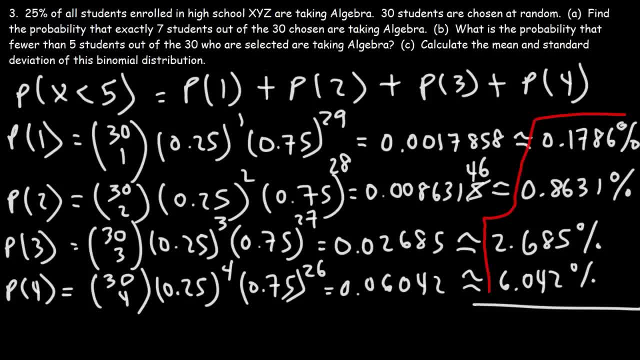 to do is add these four values to get our final answer. So that's going to be 6.042%. So now what we're going to do is add these four values to get our final answer. So the probability of getting fewer than five students who are taking algebra out of 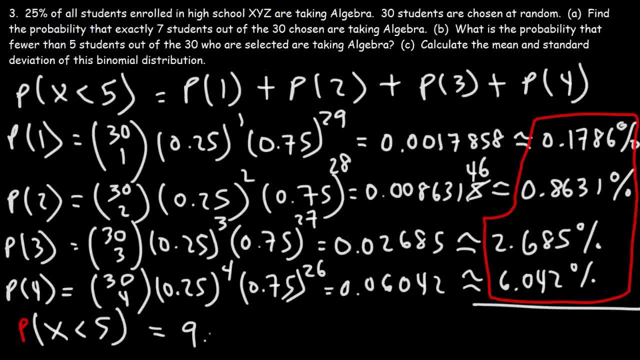 the 30 chosen, that's going to be approximately 9.769%. So if you have an inequality, such as fewer than five, you need to calculate multiple values in this case. So you have to calculate the probability of getting one, two, three or four students. 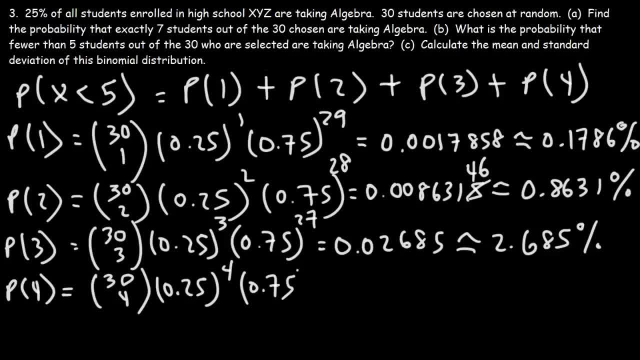 0.20875.. 0.05625.. 0.25245.. Right- 네 3 �ن. And then I have to try and find the right ratio, Which is 2.028, right And b velocity surviving. 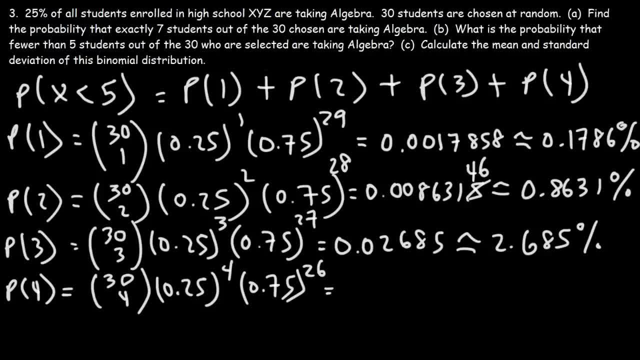 Therefore, I'm just going to calculate it by multiplying this down by 14.. And the flow rate soldier is just going to be number, though: 0.2715.. 0.03618.. 0.024.. 0.03618.. 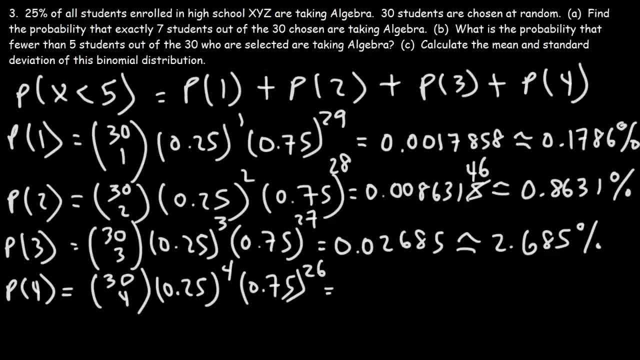 0.0213.. 0.26 007.. So now what we're going to do is add these four values to get our final answer. So the probability of getting fewer than five students who are taking algebra out of the 30 chosen, that's going to be approximately 9.769%. 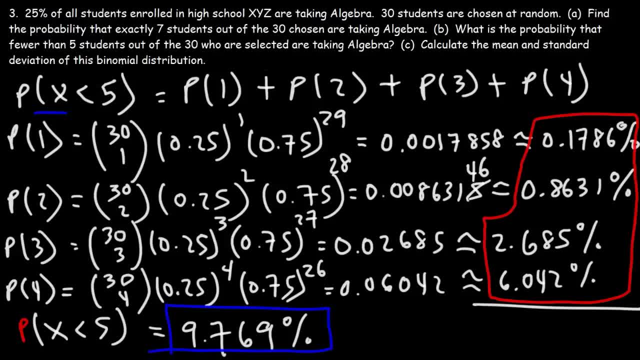 So if you have an inequality such as fewer than five, you need to calculate multiple values in this case. So you have to calculate the probability of getting one, two, three or four students out of the 30 who are taking algebra. As you can see, this could be a long repetitive process. 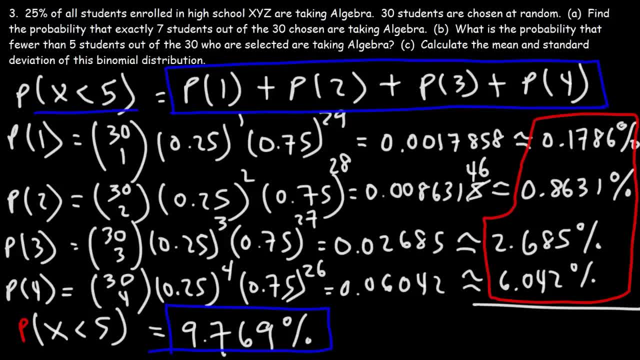 And if n is very large, you could use the normal distribution to approximate a binomial distribution. But for this particular example, since we only have to calculate four, I just decided to add all four values. Now let's move on to part C, the final part in this video. 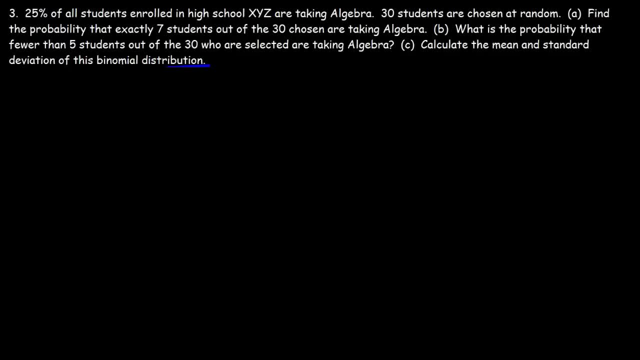 So how can we calculate the mean and the standard deviation of this binomial distribution? How can we do that? The mean is going to equal the number of trials times the probability of getting a successful event, And in this case it's 30.. 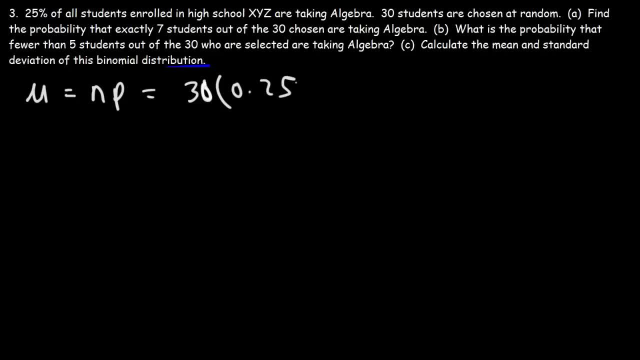 We know that p is 0.25.. So it's 30 times 0.25, which is 7.5.. So, as you can see, it's very easy to calculate the mean, The mean if you know n and p, which is given to you in the problem. 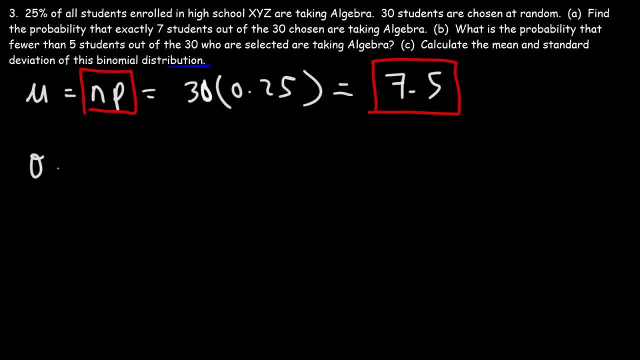 Now to calculate the standard deviation. it's not that difficult either. It's the square root of n times p times q. n is 30, p is 0.25, q is 0.75.. Now let's go ahead and plug this in.